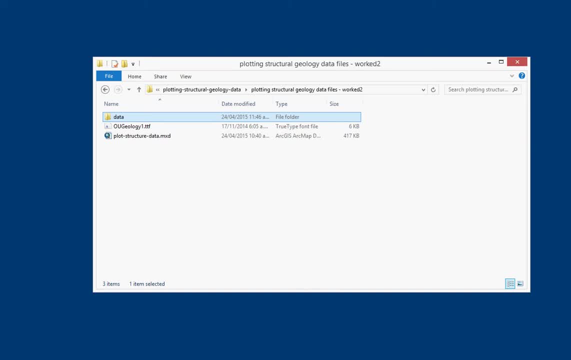 Hi there, in this tutorial I'm going to cover plotting structural geology data in ArcGIS. So this is could be foliation data, could be lineation data or any other data that we want to rotate. So to plot foliation data we need a spreadsheet with some locations and the orientation measurements. 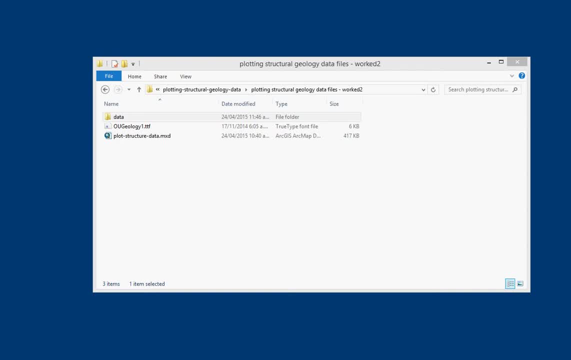 that were made at those locations. we've supplied you with some files to work through and if we look here we've got a map, we've got a font, and then this data file, data folder, we've got a spreadsheet. so I'll just open that up. 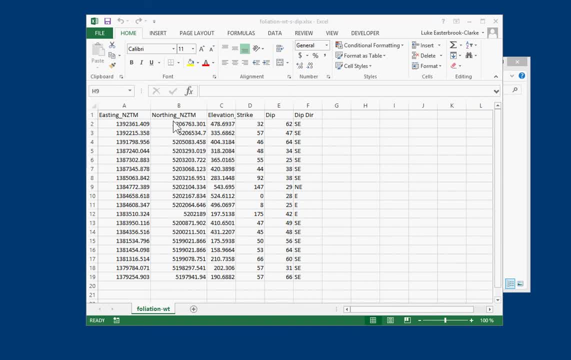 So what you can see currently is that we've got a spreadsheet so I'll just open that up. So what you can see currently in the spreadsheet is we have easting and northing elevation, but the data is in strike dip and dip direction in separate fields. Now sometimes I see people come to me with 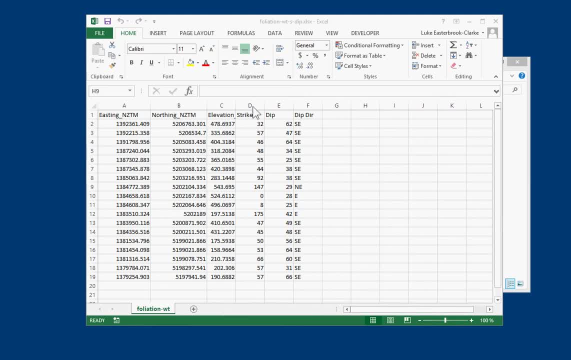 strike, slash, dip, dip direction all in a single column To convert that. I mean you really need to have those in separate columns in order to work with them. So what you can use is various Excel operations, such as mid. these are substring operations. 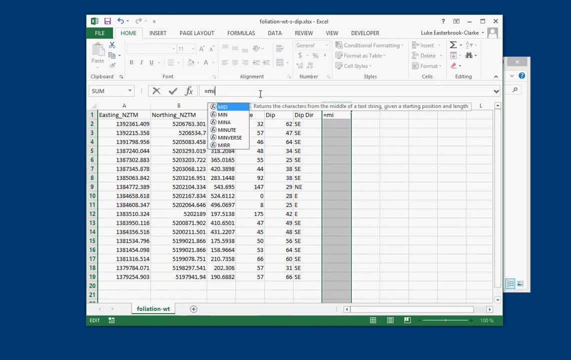 so they take a string and take different parts of it, so one is mid, another is left and another one you might need to use is right and you might have to do some manual fix up after this. So the problem with strike is the way it's structured. So if you come to me with the 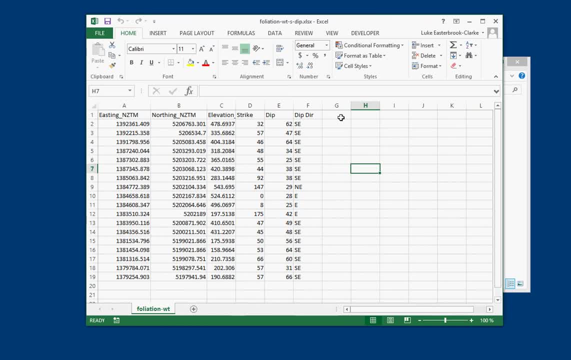 dip and dip direction is that it's not really good for a computer program that's trying to recognize it. some some software will deal with dip direction, but a lot of stuff you need to use dip azimuth and dip. so dip azimuth is the. in the case of foliation data it is the direction. 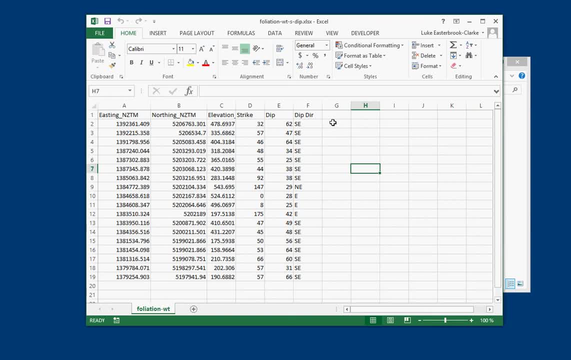 that the tick is pointing towards. so what we need to do now is to convert it. so the easiest way to convert it is to create a few different options. so I'm going to say dip, dip as one, dip as two and dip as three. so the first one, dip as one, is going to equal this. 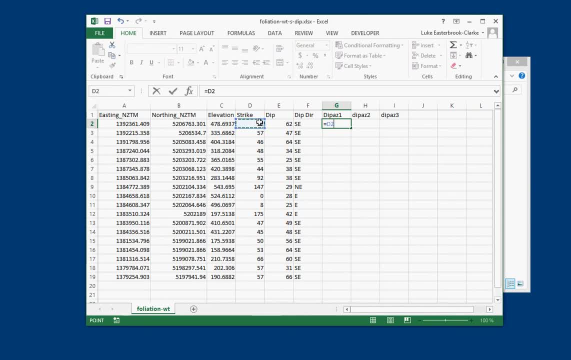 plus 90, second one is going to equal the strike minus 90 and the third one is going to equal: this equals the strike plus 270. so those are our options there for dip azimuth, and then we just basically have to look through and compare with the dip direction, decide which one is most applicable. so let's just 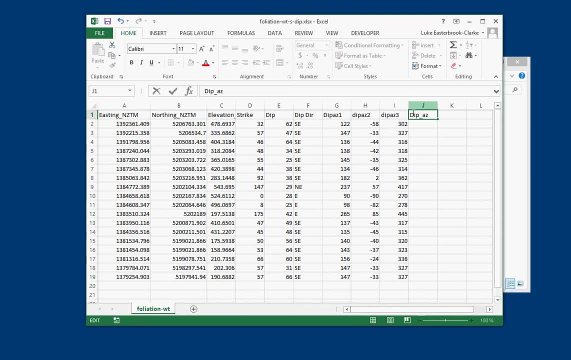 call this my to look through these three fields. another thing you can do here is if you make this one a modulo 360.. so equogz mod 260, then you don't actually need the second comment, your second column 3077 บ件. 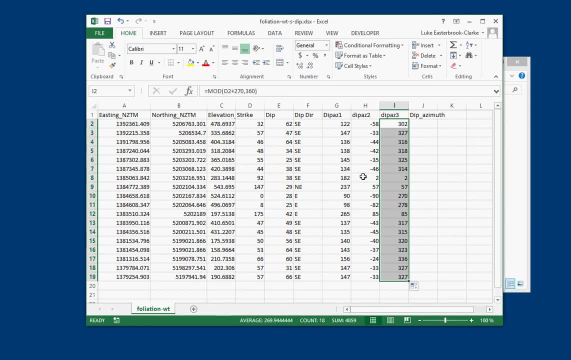 B2. that when it gets above 360, it just takes the remainder. that's what the modulo operation is, So we can delete that column, and we've just gone down to two choices now, so that 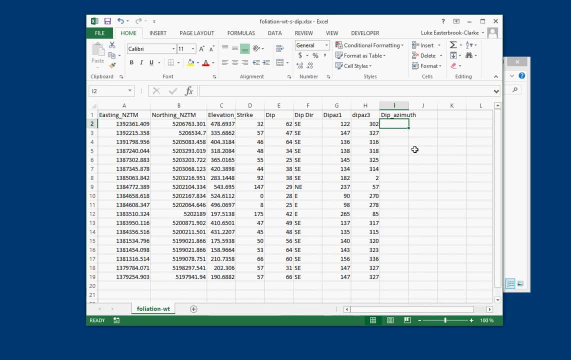 makes things a bit easier. Now you can set this up so you do equals, and if this one's empty, if this equals zero, yeah, let's do that equals. if- sorry- if logical test is that equals zero, then it should be this one, and then if that's not true, then it should. 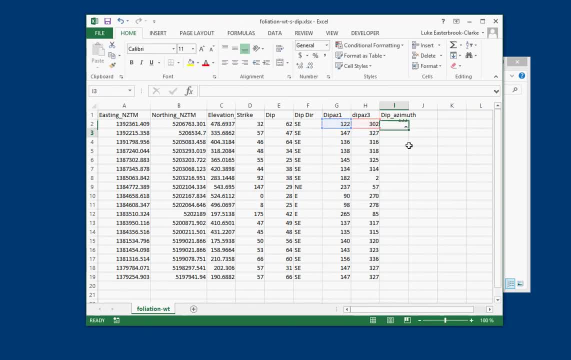 be that one, and then we can just delete the one we don't want. So let's fill that down. so this one, it should be 122, that's southeast, that's southeast, southeast, southeast, southeast, and this one is well, it should have been south actually. 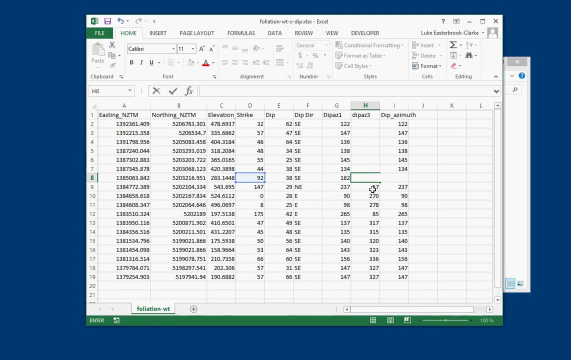 see, this is why this is sometimes problematic. This one here is northeast, so it is not that one, because this is northeast quadrant. This one here is east, so it's the 90, and this one here is east as well. and this one. 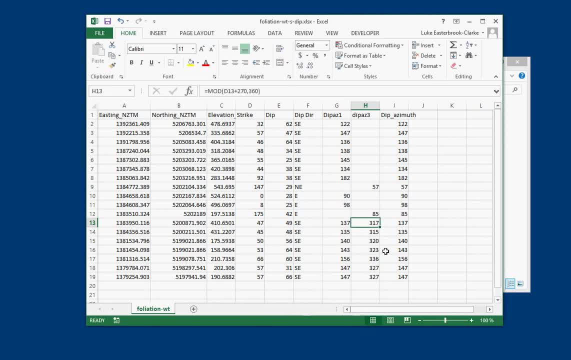 here is east, so we delete that one and then all the rest of these are southeast. Now it's kind of nice here to we can copy and paste and this is values, because we don't want any of these sort of workings. 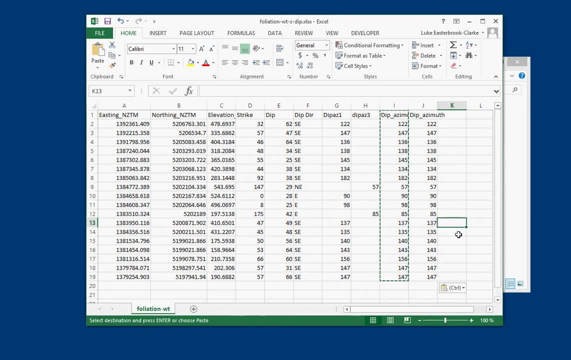 You can copy and paste, and this is values, because we don't want any of these sort of workings. You can store them, but we kind of need, want to keep things simple, so we can get rid of all four of these fields now and let's also let's actually paste those ones over. 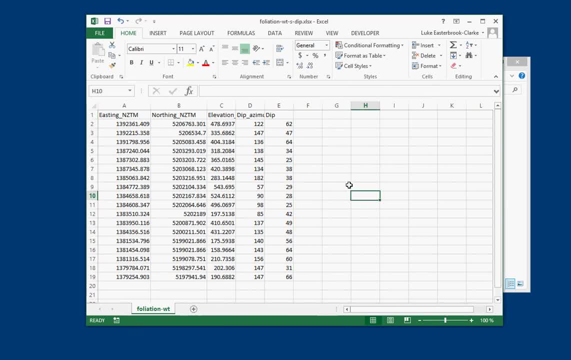 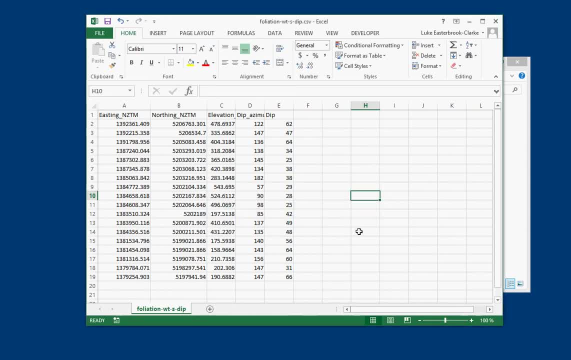 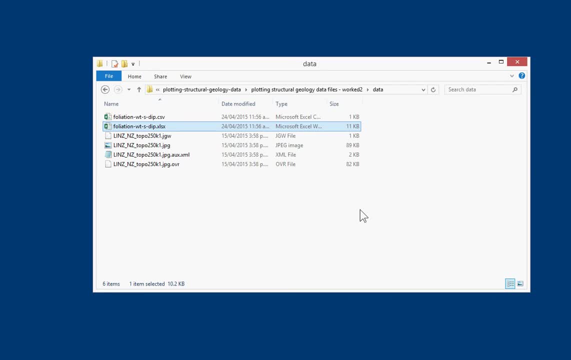 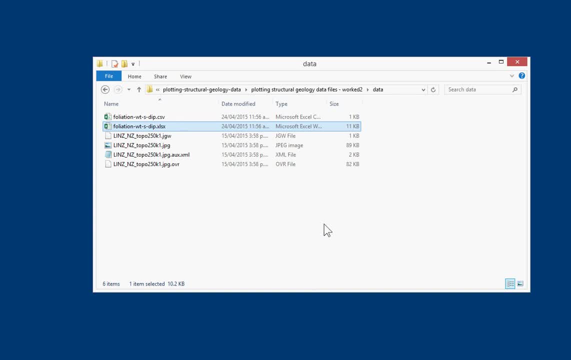 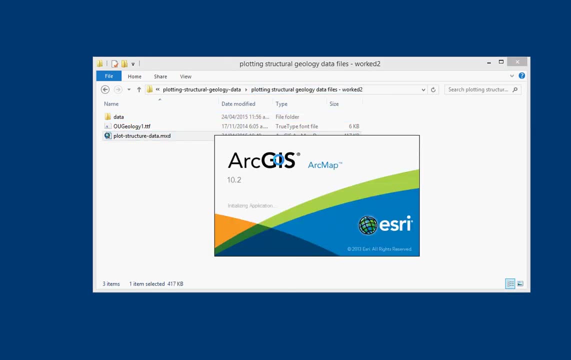